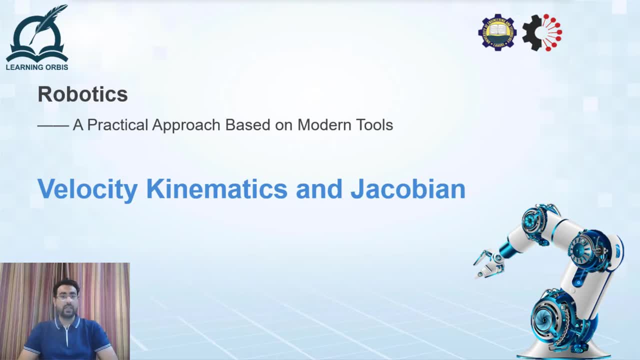 If you have viewed the previous video that was of trajectory generation, then you must remember that trajectory doesn't only include the end-effector's position information, It also includes its velocities and acceleration information. So if the robot is following a particular trajectory, then it means it should be following the position, velocity and acceleration profiles of that trajectory. 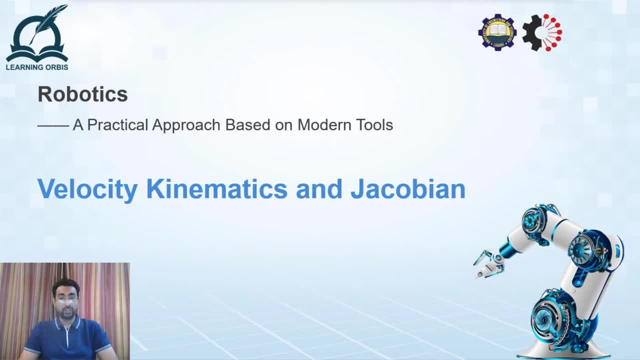 Till now we know how to convert joint angles into end-effector positions and vice versa, ie end-effector's position into joint angles. But do we know how to convert joint velocities into end-effector velocities and vice versa? 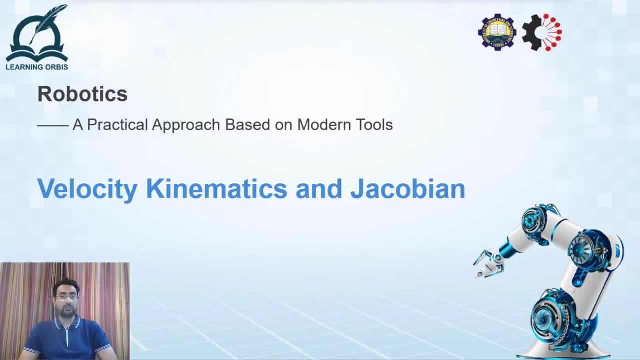 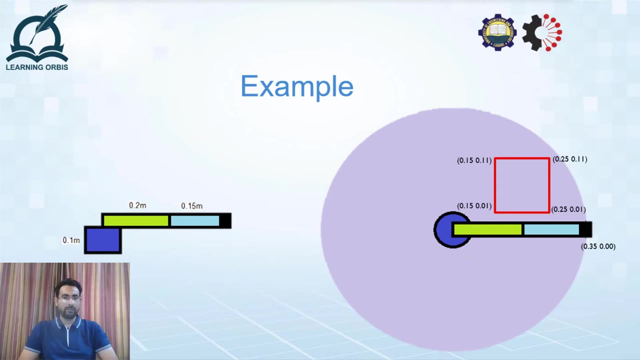 Well, this is the topic of this video. We are going to extract a transformation matrix, famously known as the Jacobian, of a tripotic manipulator that will transform the joint velocities into end-effector velocities. For this video, once again, I am going to use a simple 2 degree of freedom planar manipulator that we have designed in the previous videos, and I am going to drive it on a square trajectory, as shown over here. 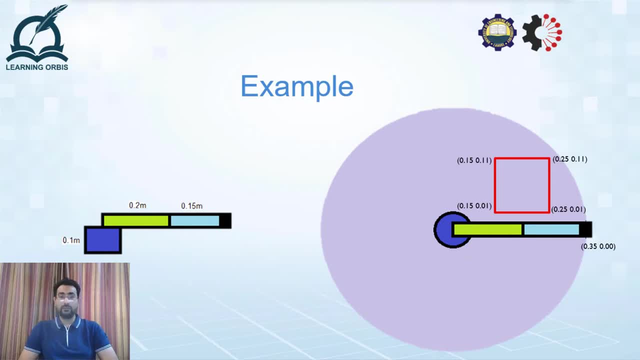 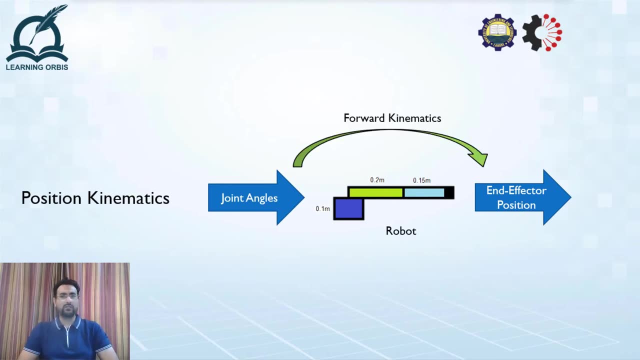 If you are not sure how to drive the robot in this trajectory, kindly view the previous video related to trajectory generation. Well, just to revise a bit, we have covered position kinematics, in which forward kinematics will transform the joint angles into end-effector positions and inverse kinematics will transform end-effector positions back into joint angles. 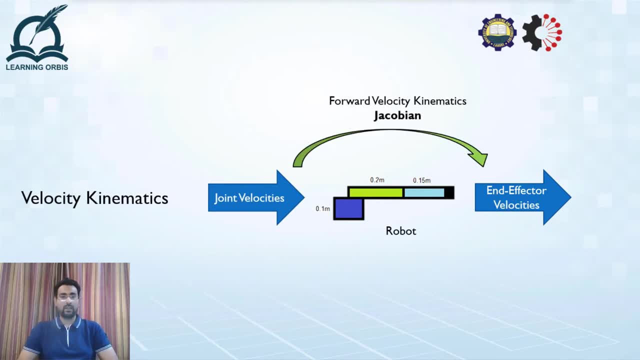 However, today we are going to implement velocity kinematics, in which the matrix Jacobian will transform the joint velocities into end-effector velocities, and inverse Jacobian can be used to figure out joint velocities given the end-effector velocities. So, without any further delay, let's jump to the Simulink environment and see how we can extract a Jacobian using Robotic System Toolbox. 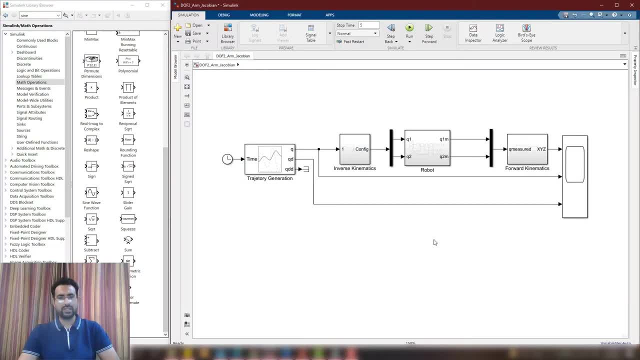 and use it to perform the velocity kinematics beyond the. So this is the Simulink model that we used in our previous video of trajectory generation. Over here at the start we we're generating trajectory, providing that trajectory to the inverse kinematics block. 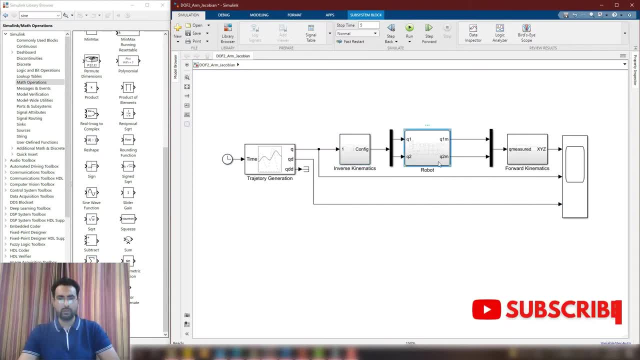 The inverse kinematics block was converting that trajectory into joint angles which were being provided to the robot over here. Then we were measuring the joint angles of the robot, providing those joints angles to the forward kinematics, And forward kinematics will convert the joint angles back into the end-effector positions or the trajectory. 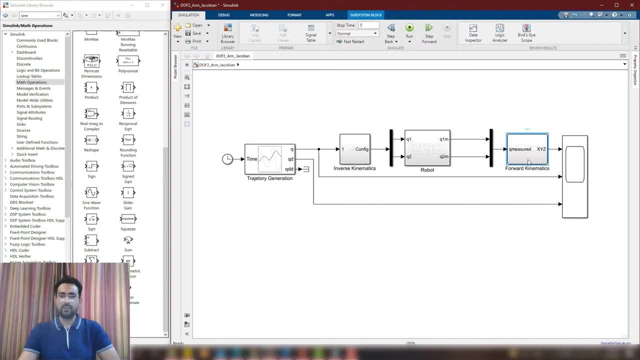 Then we will compare this attribute to the forward kinematics, as in the quadratus over here, over here, planar degrees is 0, 0, 0, 0, 0, 0.. Here you go, the trajectory on which the robot was moving with the trajectory that we were. 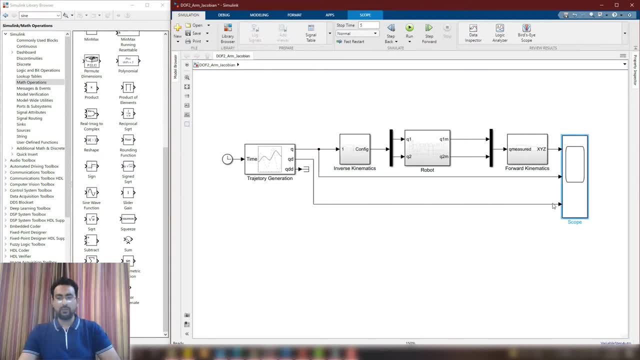 providing using this scope. Along with the position information, we were also viewing the velocity of the end-effector as well. But are we sure that, whatever the velocity we were providing to the robot, the robot was moving on that same velocity? Well, today we are going to see that. For that we will be needing a 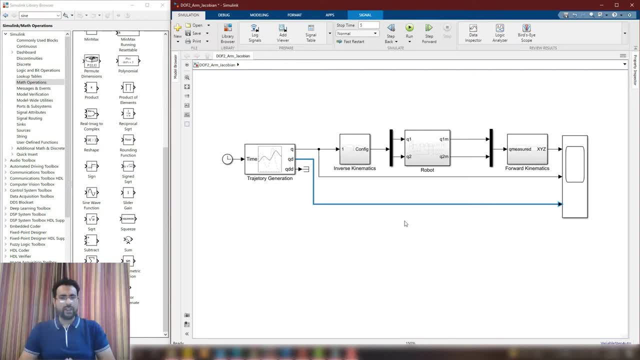 number of things which I am going to explain step by step. So the very first thing we need is we need to get the Jacobian matrix. That is the matrix that is going to transform the joint velocities into end-effector velocities. So once we have that matrix, we are going to multiply that matrix with the joint. 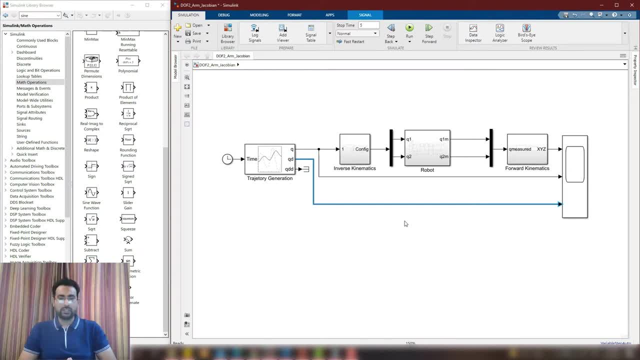 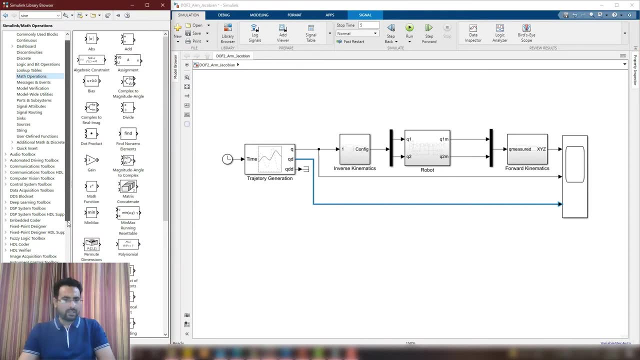 velocities and then it will give us the end-effector velocities So that we can compare the end-effector velocities with the trajectory velocities. So let's get started. If you will come in the robotic system toolbox and then, under manipulator algorithms, you will see a block named as get Jacobian. So it is the. 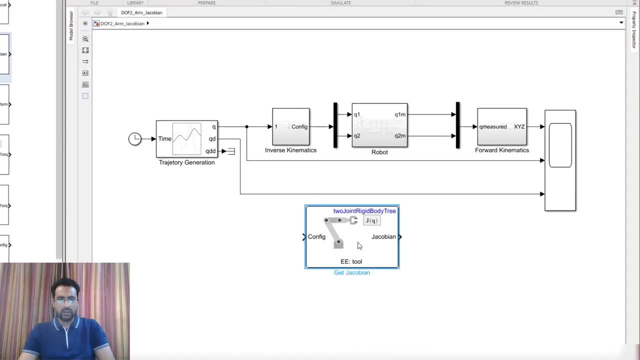 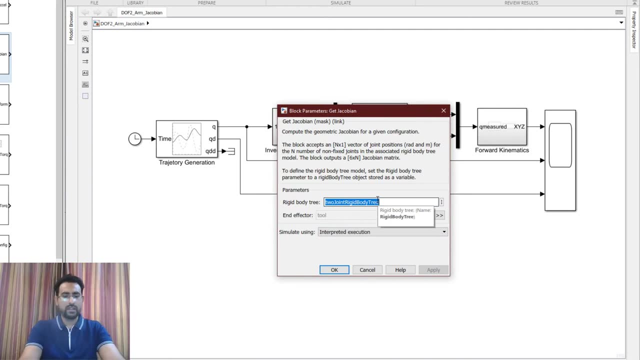 simplest way to get the Jacobian matrix. I'm going to drag it over here. I have to provide this block with the rigid body tree of my robot. So just double click on it, go into the settings and write a variable which contains the rigid body tree of our robot. Make sure. 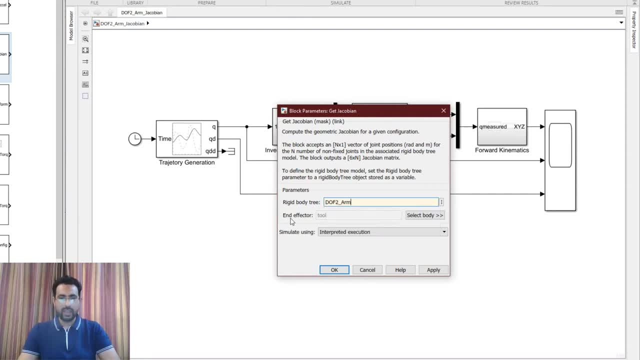 that you have loaded this robot into the workspace. The second thing is we have to select the end-effector. So for that, I'm going to click on the select body, and the last body is my end-effector. So I'm going to select it and that's it Now. 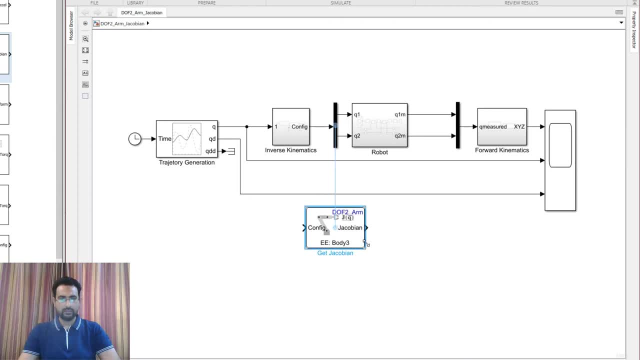 this block is going to provide me the Jacobian matrix. Let me just resize it. I have to provide the configuration, that is, the joint angles to it. I have this configuration over here and on the other side it is going to give me a Jacobian. This Jacobian will be a six cross n. 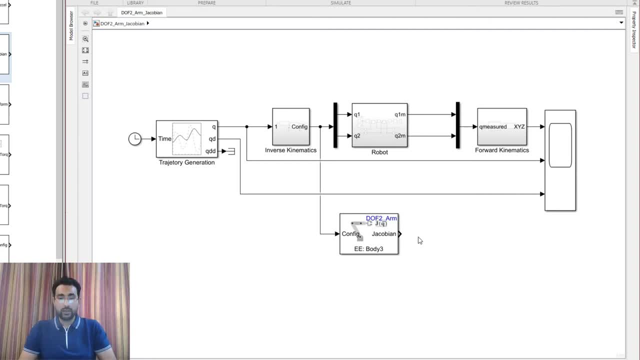 matrix Six is coming from the six velocities we are going to get. The first three velocities will be the angular velocities, whereas the last three velocities will be the linear velocities. Sometimes in literature the arrangement is opposite, That is, the upper three velocities or the first three velocities. 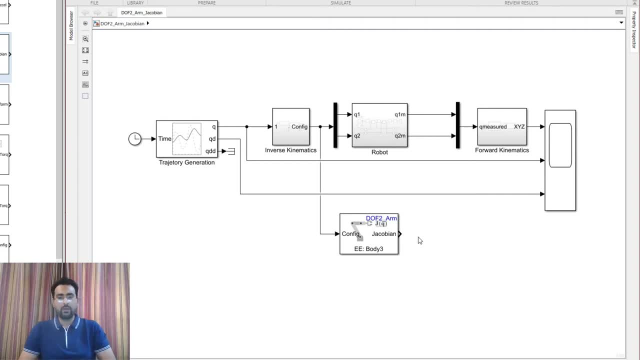 are the linear velocities and the last three velocities are the angular velocities, Whereas in MATLAB robotic system toolbox the order is reversed and the columns of this Jacobian matrix will correspond to the number of joints we have. So right now we have two joints, that is, we have two degrees of freedom. 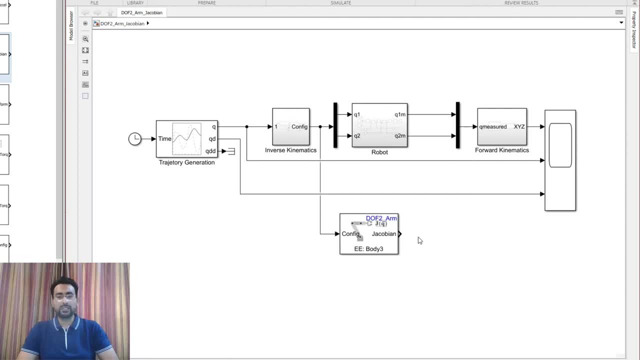 robotic manipulator. so we are going to get a Jacobian of 6 cross 2.. So now all we have to do is we have to multiply this Jacobian with the joint velocities. but right now we don't have the joint velocities, So for that we have to go. 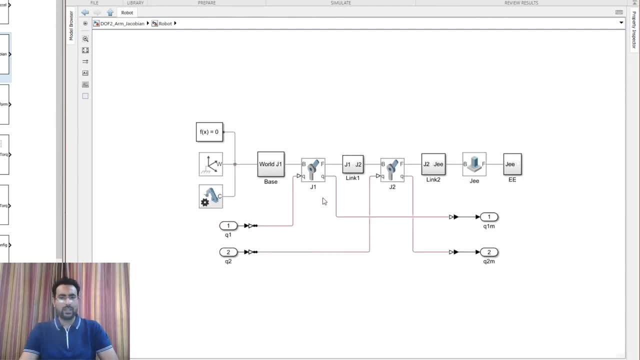 into the robot and we have to sense the joint velocities exactly in the same manner. we are sensing the positions of the joints, So we have to go into the joint one and then in the sensing portion I'm going to check this velocity. so now I'm going to get a velocity over here. 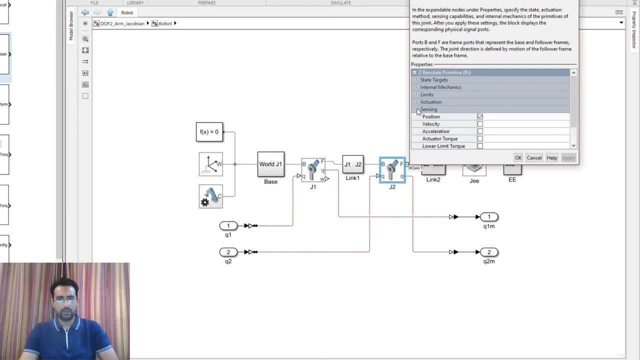 which is shown by this W port. Similarly, for joint 2, I'm going to sense the velocity and I'll get the W port over here as well. so to get these two velocities out of this block, I need two output ports. I'm going to use these two ports. I'm going to name them as: 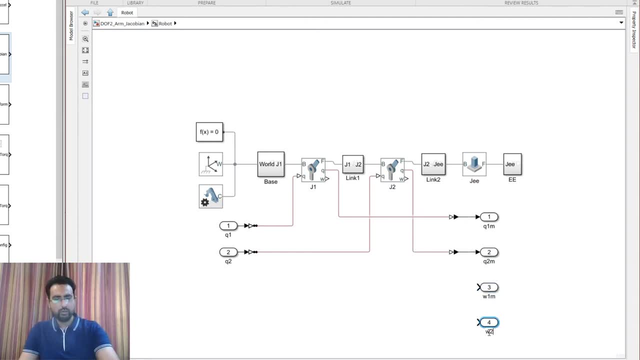 W1 measured and W2 measured, and I'll use a PS to Simulink converter over here and over here as well. so that's it. I've connected the joint 1's velocity with this 3 number port and joint 2 velocity with this 4 number port. Now on this side you can see that we have two. 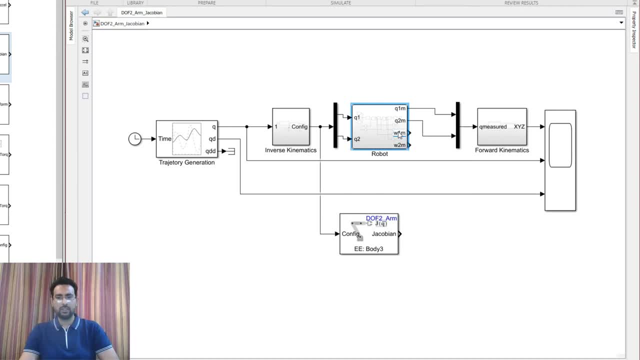 more ports. W1M and W2M. that is the measured velocity of joint 1 and joint 2.. We have to multiply these velocities with the Jacobian, and for that we need to first mux them together so that we can have one matrix of velocities. 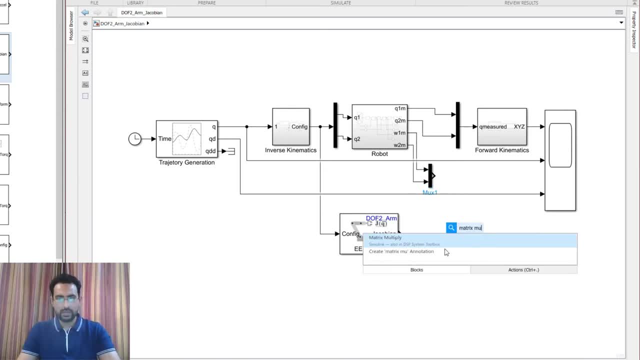 and for matrix multiplication, I'm going to use a block of matrix multiplier. the first matrix will be the Jacobian and the second matrix will be the vector of velocities. So that's it. Now. on this side, I will be getting six velocities related to my end-effector. 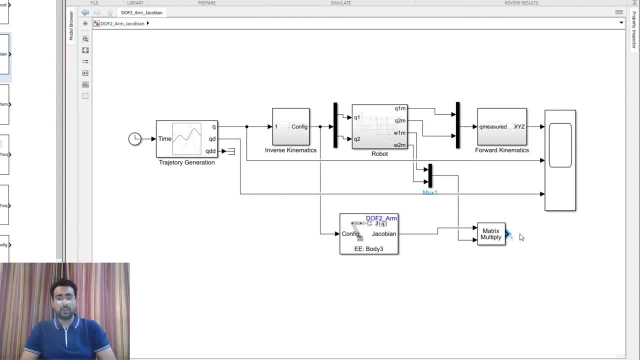 out of these six velocities, first three will be the angular velocities of the end-effector and the last three velocities will be the linear velocities of my end-effector, as we are not concerned with the angular velocities right now, so I'm going to terminate them, whereas for the linear velocities, I'm going to compare those linear velocities. 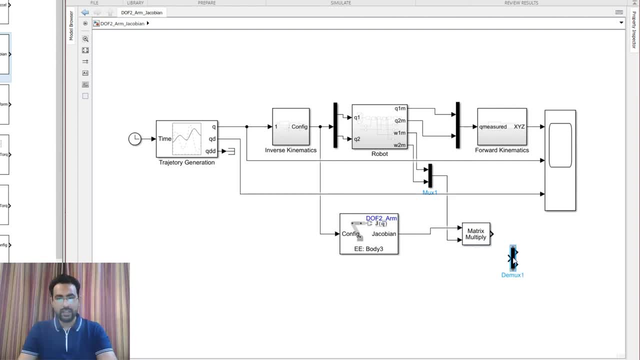 with the linear velocities of the trajectory, so I have to divide them into two portions: the upper half and the lower half. The lower half are the linear velocities and the upper half is the angular velocity. I don't need the angular velocities, so I'm going to terminate them. 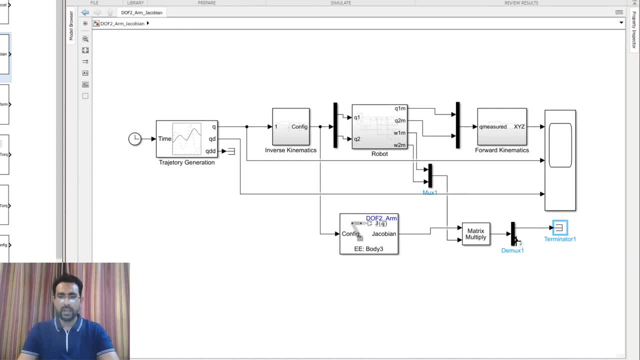 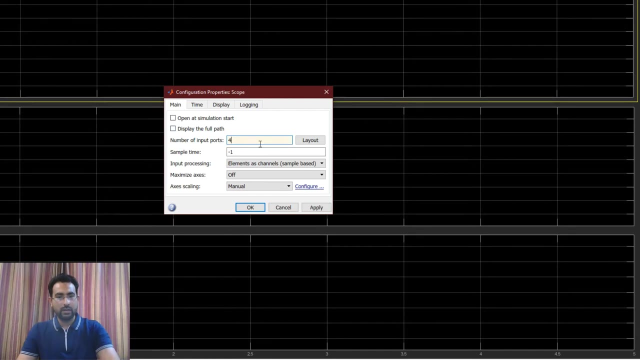 using a terminator and I will be providing the linear velocities to the school so that we can compare the end-effector velocities with the trajectory velocities which we are already providing. So for that I need one additional port in the scope. I can get that port like this: Now I need four ports and I'm going to change the. 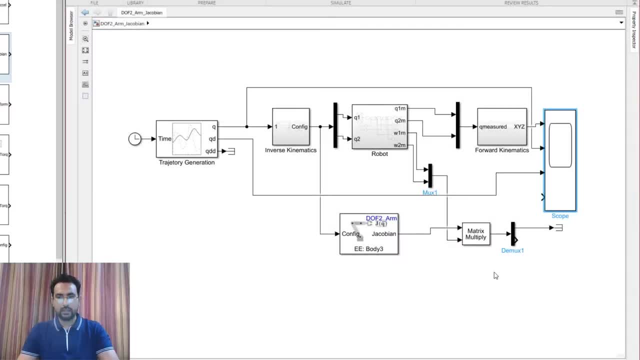 layout into this side 2x2 layout. so over here I'm going to provide the end-effector velocities. so this is essentially everything we need. now we just need to run this simulation and see that, what end-effector velocities we are getting by using Jacobian and what end-effector velocities we were providing. 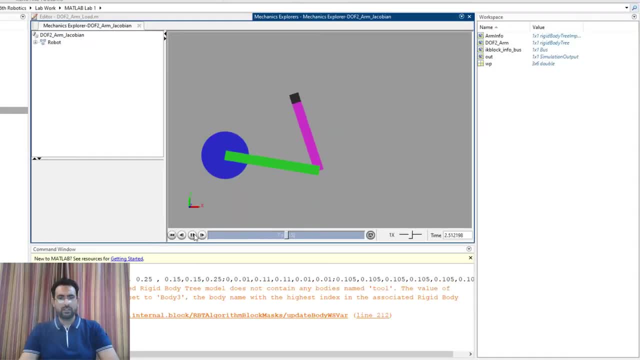 to the end-effector velocities. So this is the simulation we are getting. you can see that our robot is moving on the trajectory quite nicely, as we have specified the trajectory, but what are its velocities? we don't know about that. so let's have a look at the 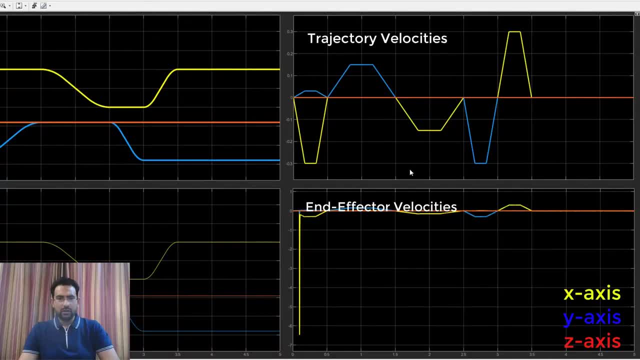 scope and see that. what are the velocities? So here we are. this graph shows the velocity that was of the trajectory that we wished our robot to follow, whereas this is the velocity which our robot is following. You can see a discrepancy over here, which is because, at the very start, the inverse kinematics- 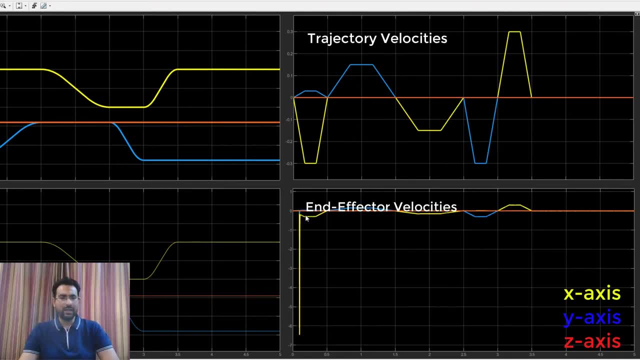 couldn't find a solution, but that's the reason why we are using this simulation. So after a certain time, it suddenly finds a solution and the end-effector abruptly jumps to that solution. therefore, we have a huge velocity at the start, whereas after that the things get normal. 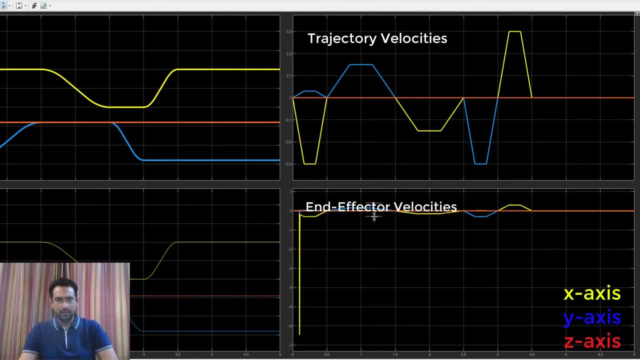 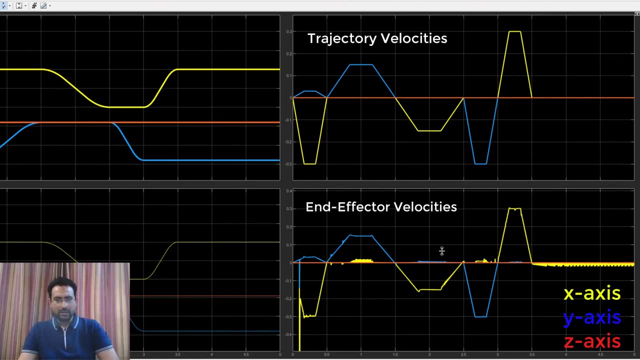 So let me zoom a bit so that we can compare the velocities of the trajectory and the velocities of our end-effector. You can see that the overall shape is quite fine, but there are certain errors in the velocity. Can you figure out that? why we are getting these errors? 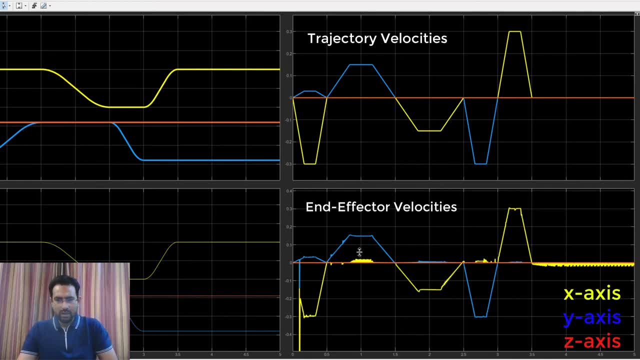 You can see that there are some errors over here. over here and in fact in all the segments we are getting some errors. If you ponder on this point a bit, then these errors are because of the errors which are being generated by the inverse kinematics block, As the inverse kinematics block is using a numerical solution to find the 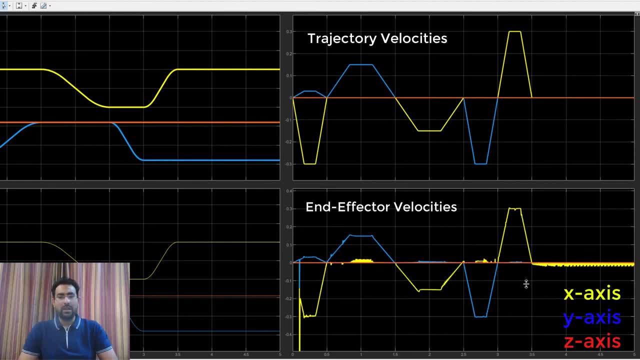 joint positions. that numerical solution will be as best as we have specified. If you want these errors to be gone, you can specify a tight tolerances and see that these errors will be reduced quite a lot. but there will be a side effect of that: the simulation is going to take much longer.